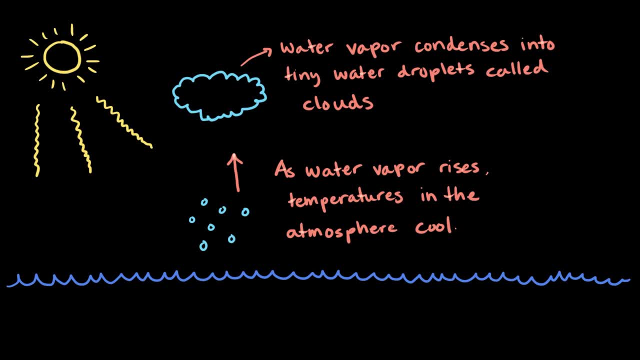 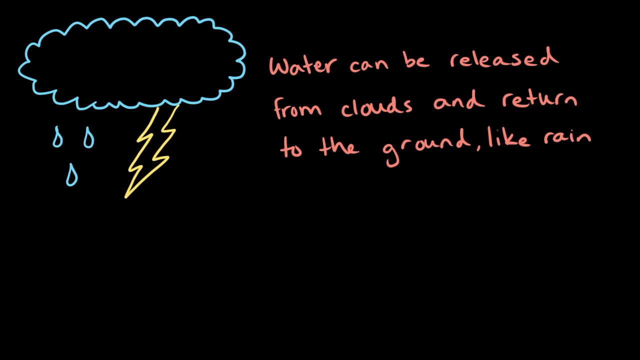 than liquid water. So the water vapor condenses into tiny liquid water droplets or, as we see them, clouds. This is called condensation. Air currents then move these clouds all around the earth. As a cloud collects more and more liquid water droplets, the water may be released from. 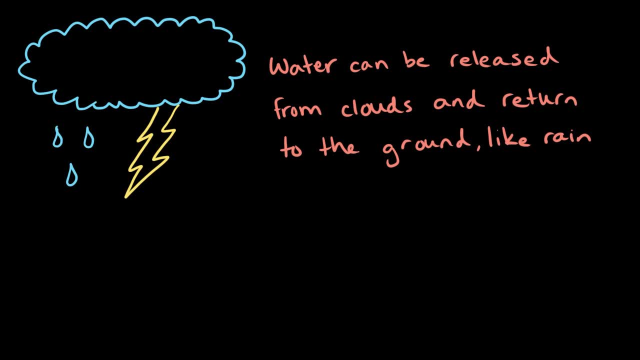 the cloud pulled down by gravity and then returned to the ocean or land as precipitation, like rain. If it's really cold, though, the water drops may crystallize and become snow. The snow will fall on the surface of the ocean and the water drops will fall on the surface of the ocean. 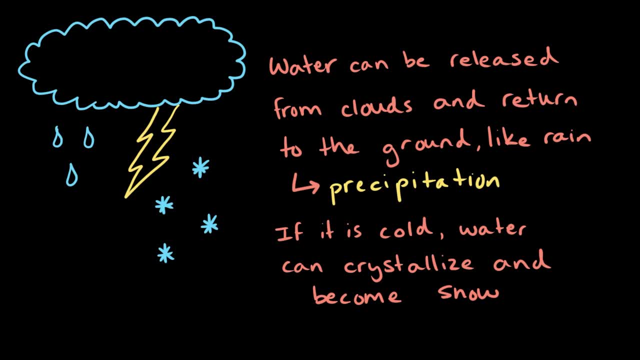 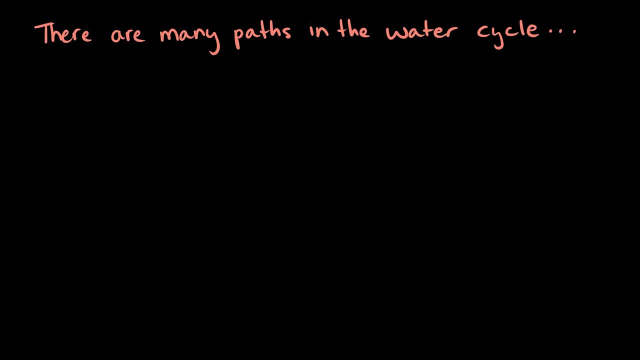 and eventually melt back into a liquid and run off into a lake or river, pulled down by gravity, which flows back into the ocean, where the whole process starts over again. But that's just one path water can take through the water cycle. It's like a choose-your-own. 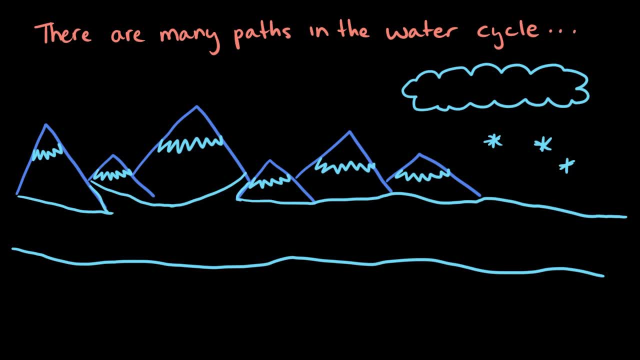 adventure. Instead of snow melting and running off into a river, the snow could become part of an icy, cold glacier and stay there for a long, long time- for thousands of years- Or rain can seep into the ground and become groundwater. 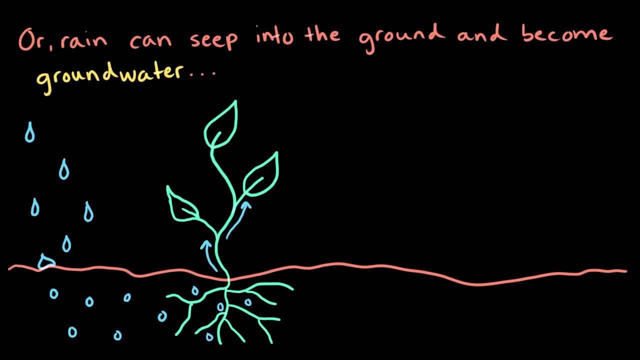 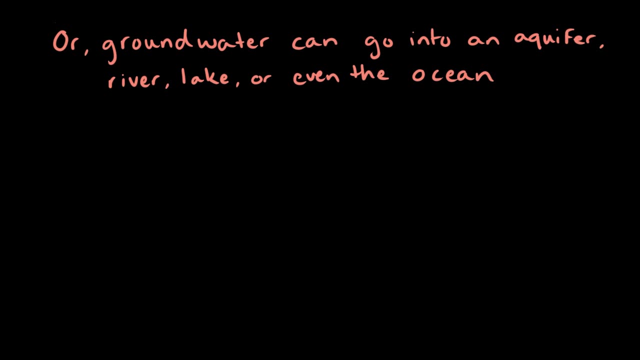 where it's then absorbed by plant roots. In turn, through transpiration, the water absorbed by the plants can transition to water vapor and leave directly through the leaves via tiny holes called stomata, and return to the atmosphere Or instead of being absorbed by plant roots. 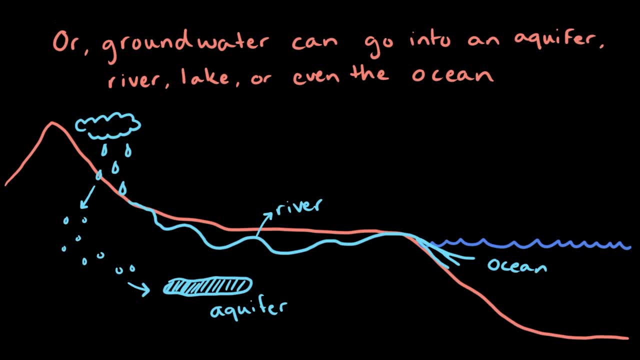 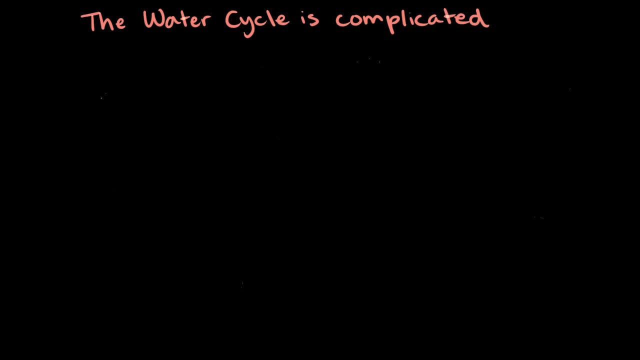 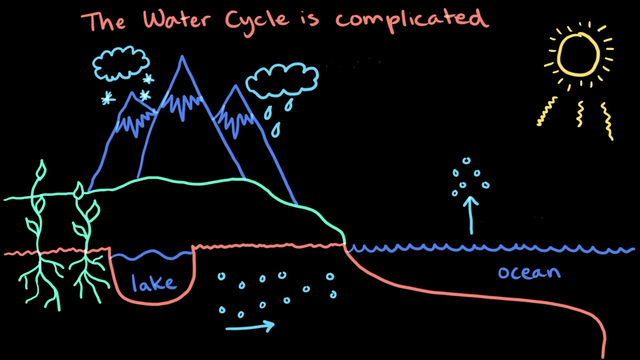 the groundwater can work its way to an underground aquifer or a lake, river or river or even river, or even the ocean. There are many different paths for water and the water cycle can be very complicated, but it really comes down to something very simple: The amount of water on earth stays. 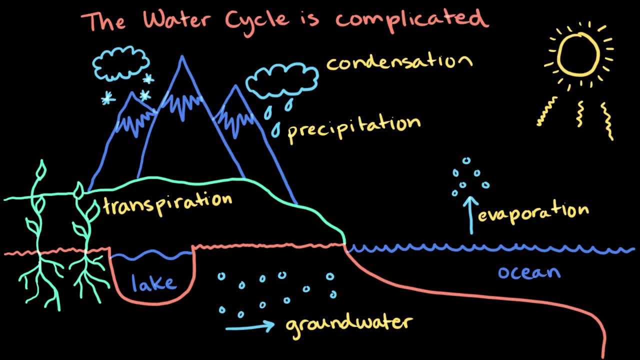 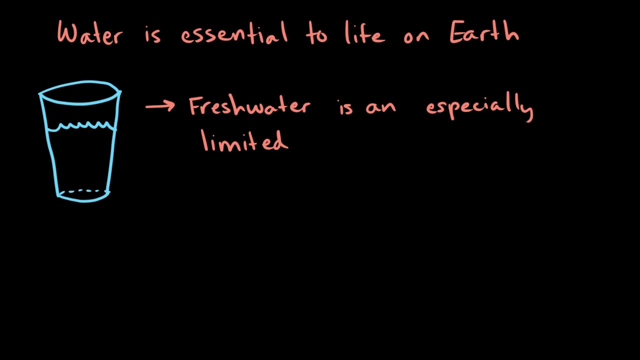 pretty constant over time and moves from place to place, sometimes transitioning between phases, depending on things like weather, geography, solar energy and gravity. Now we know that water is essential to life on earth, and fresh water is an especially limited resource for a 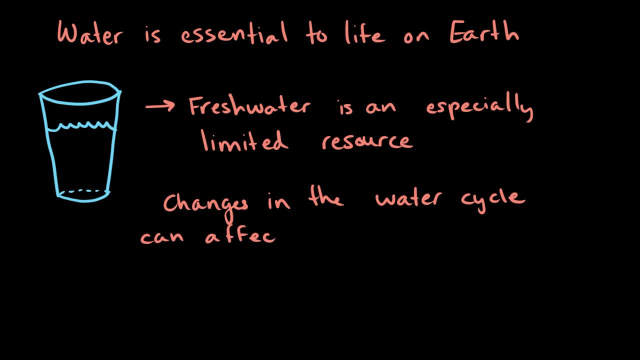 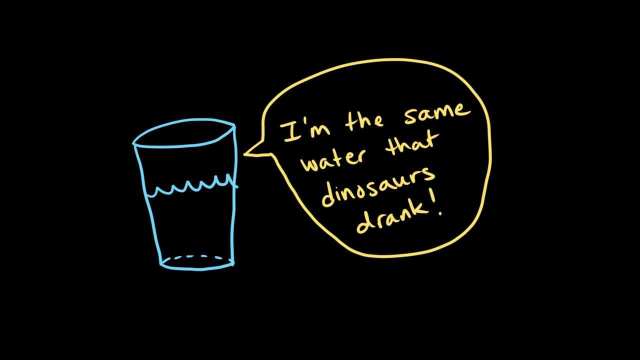 growing world population. Changes in the water cycle can impact everyone, through the economy, energy production, health, recreation, transportation, agriculture and, of course, drinking water, And that's why understanding the water cycle is so important. That, and it's pretty. 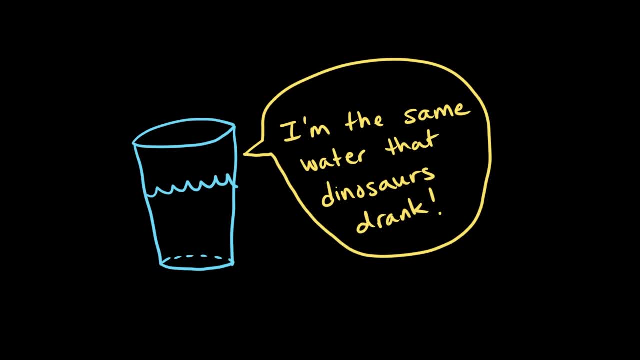 cool to know that you drink the same water as dinosaurs did. Until next time.